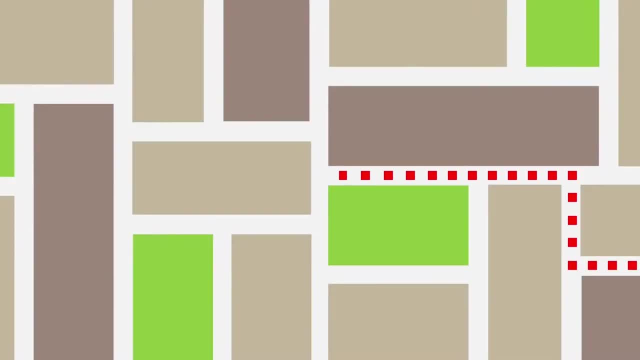 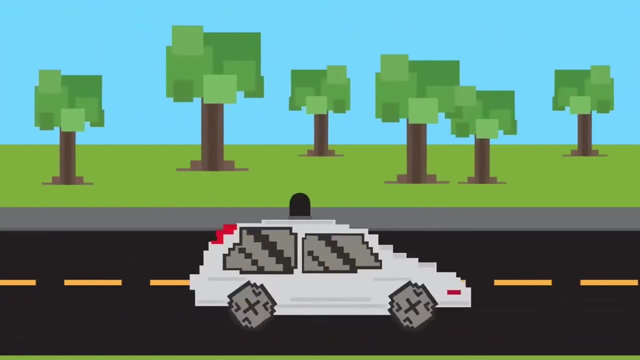 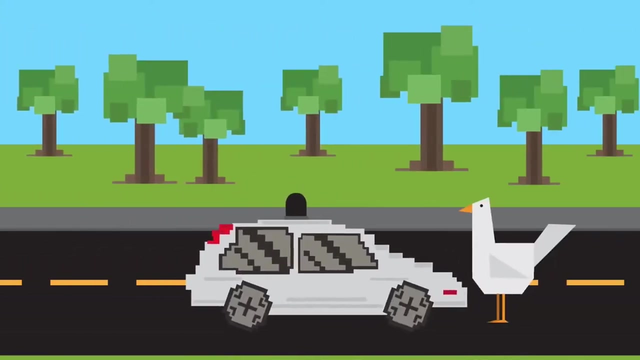 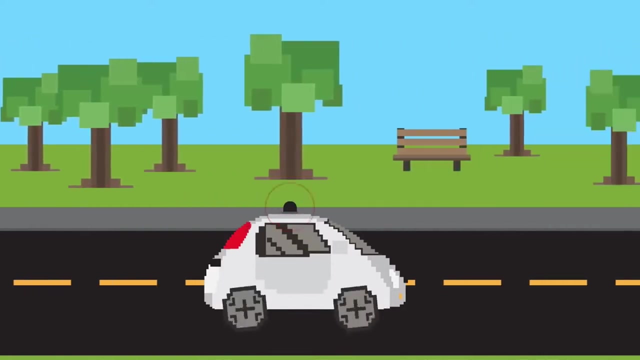 Path planning for autonomous vehicles enables self-driving cars to find the safest, most convenient and most economically beneficial routes from point A to point B. Finding routes is complicated because of the static and maneuverable obstacles that a vehicle must identify and bypass. After the route planner generates a path through the road network, the technology evaluates the surrounding environment and generates the most appropriate path for the trip. 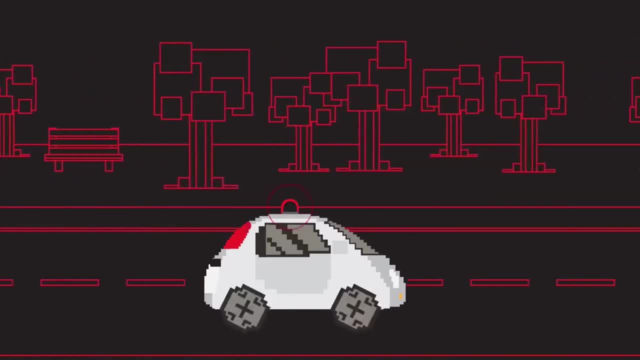 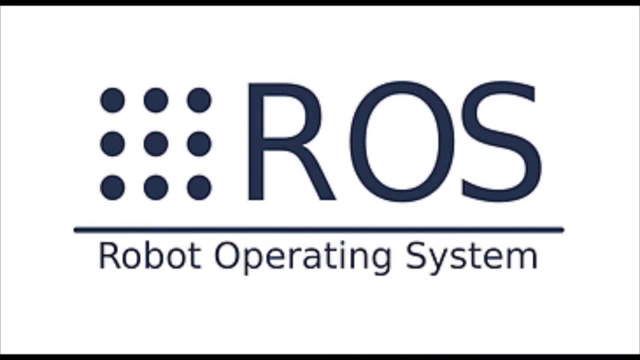 Finally, the feedback controller adjusts the mode in real time to control the route To correct errors and overcome obstacles on the road. ROS is an open source framework or a middleware software that helps in the management of various softwares and packages. It's a software environment where individual pieces of software or nodes communicate and work together. 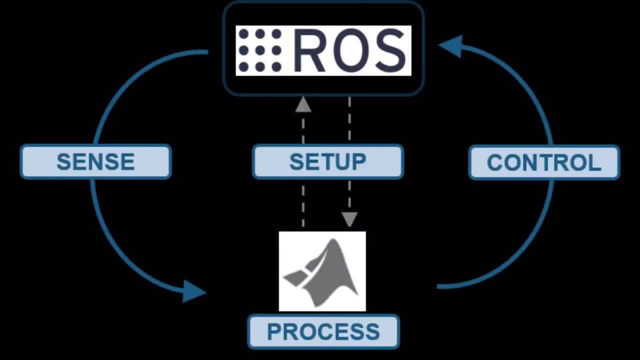 This helps in the breaking down of a huge task of a single robot into various smaller tasks, such as sensing the wall or driving the motor, Thus making the software development of a robot more effective. In addition to that, we have used Gazebo. 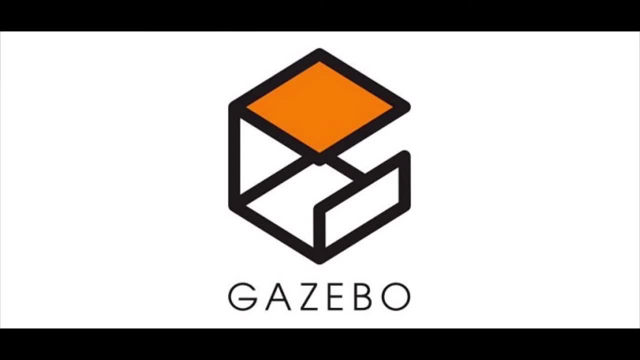 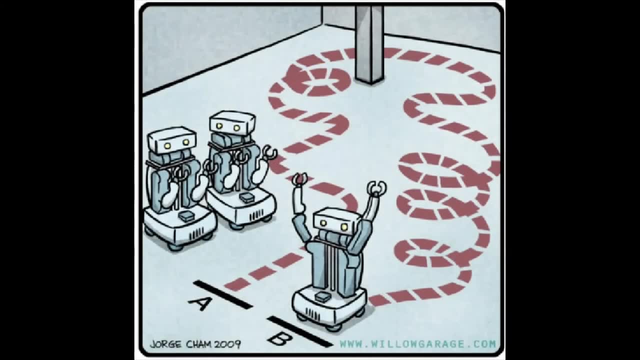 which is a 3D dynamic robot with the ability to accurately and efficiently simulate many robots in complex indoor and outdoor environments. We use the Gmapping package of ROS, which works on the principle of simultaneous localization and mapping algorithm that allows a mobile robot to build a map of its surrounding and know its location on the map simultaneously. 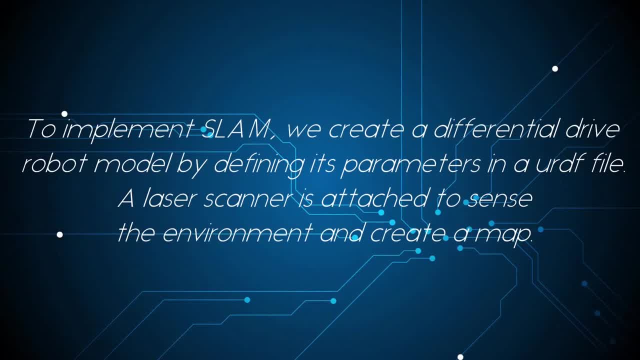 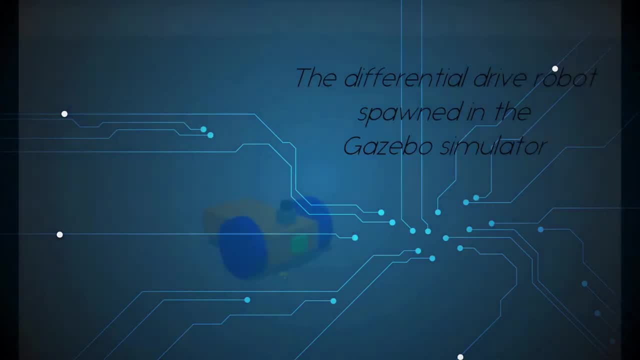 To implement SLAM. we create a differential drive robot model By defining its parameters in a URDF file. a laser scanner is attached to sense the environment and create a map. We then narrowed down the map to make it easy to see the inside and out. 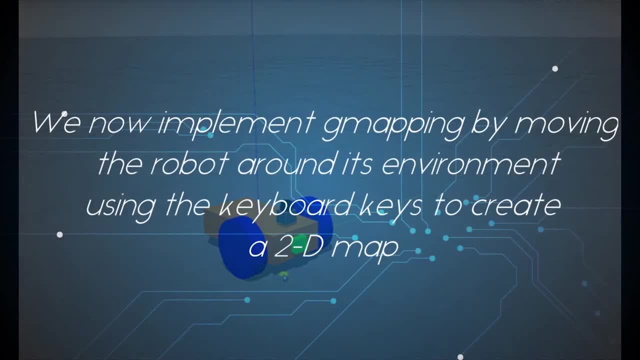 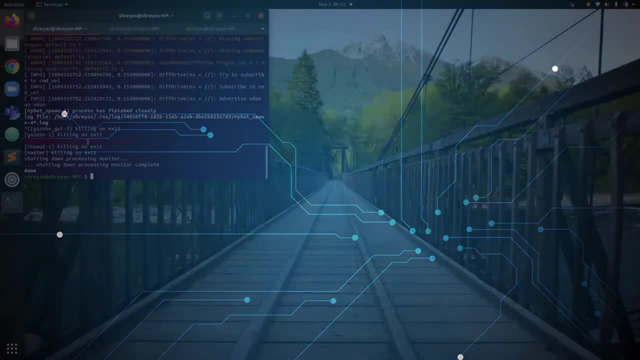 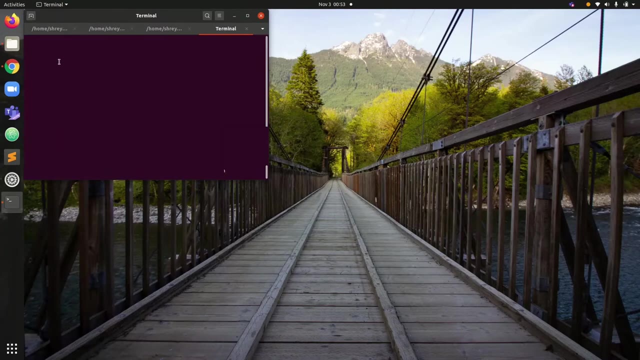 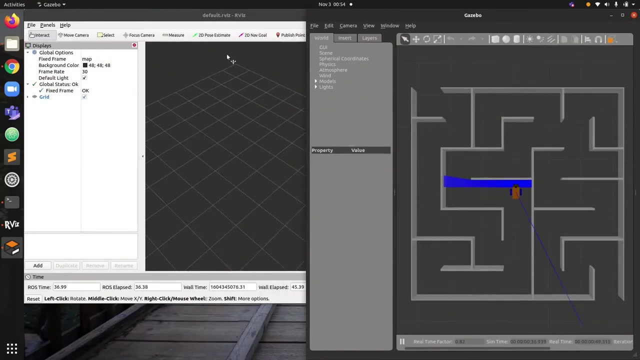 There are multiple different maps for this. This is an image of the map. The map of the map is a special complex. The map is arranged in a layout of a 3D map. The map is a 3D map. The map is a 3D map. 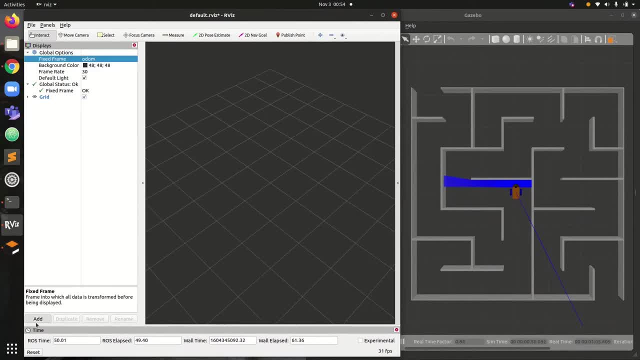 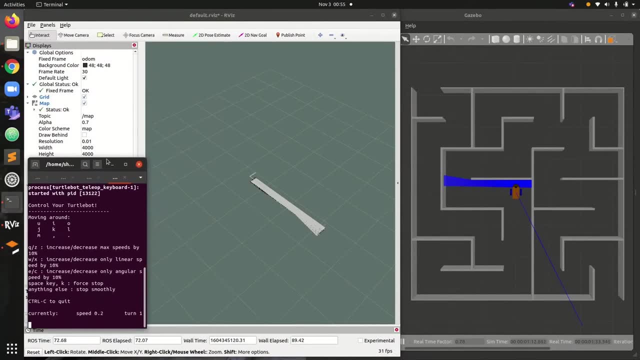 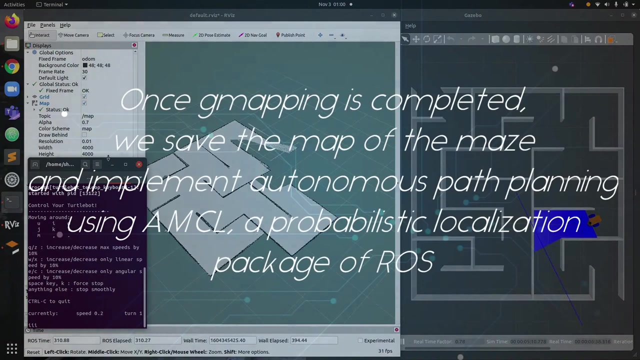 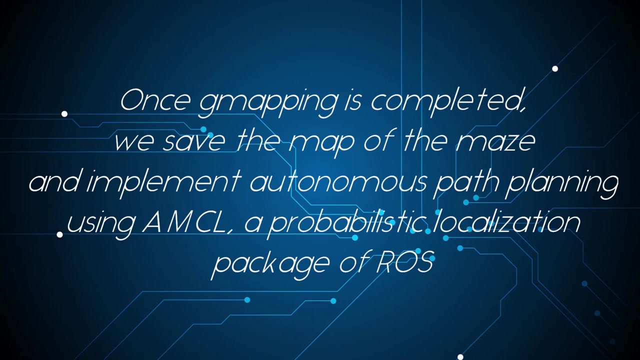 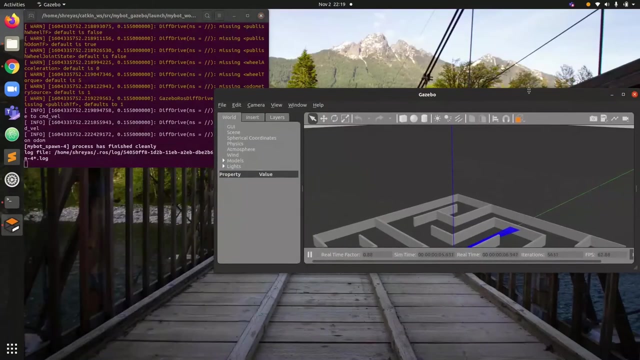 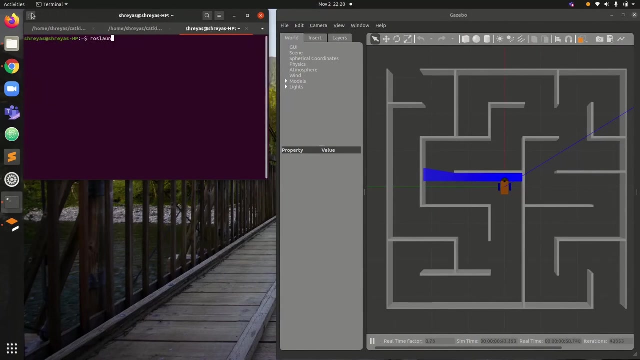 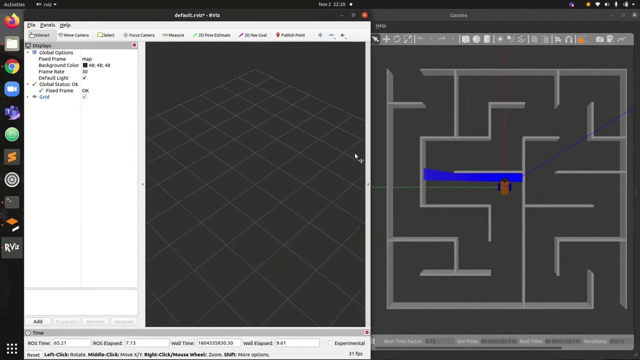 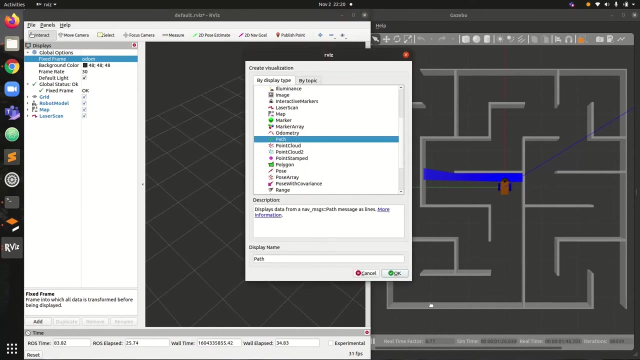 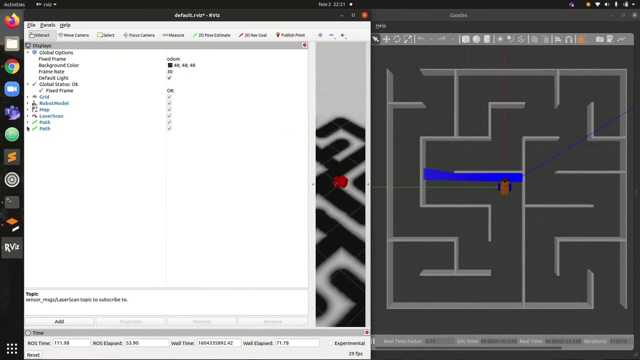 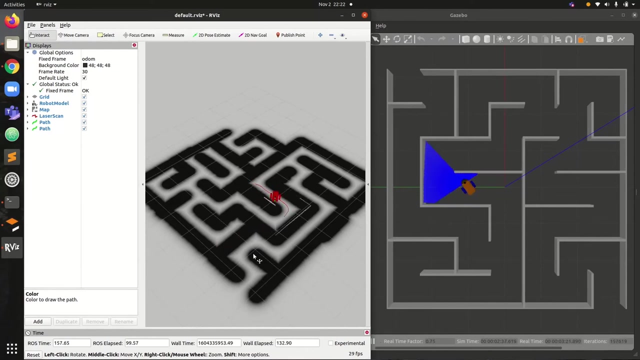 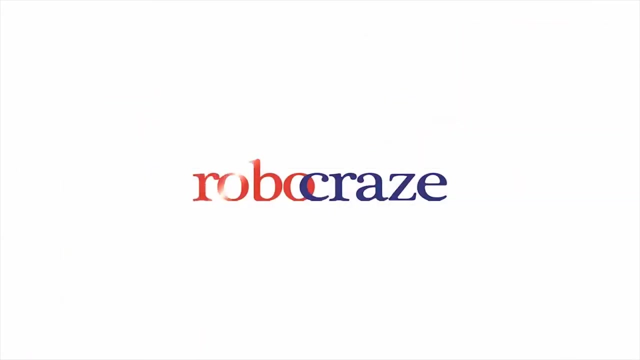